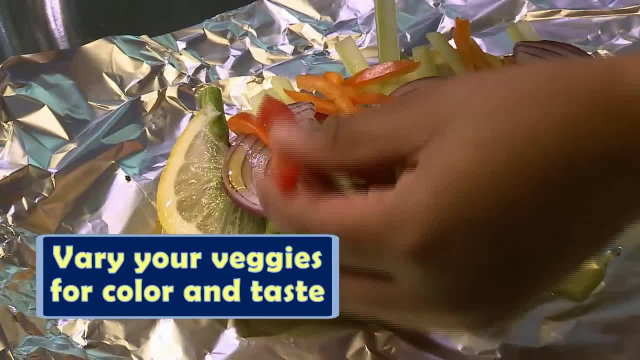 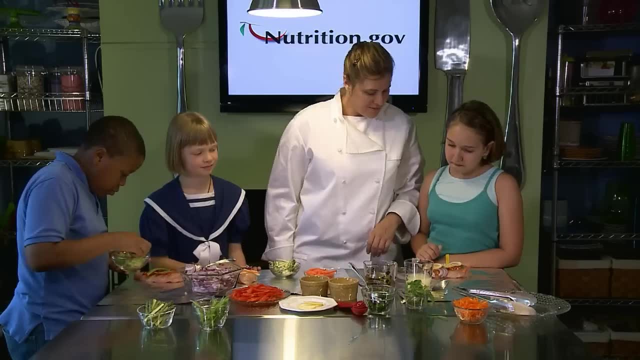 Why not try something new? Or, if you prefer, pick your favorites today and the next time you make it at home, you can try something different. These are looking good If you're making this at home with your family and everyone wants to make it their own way. 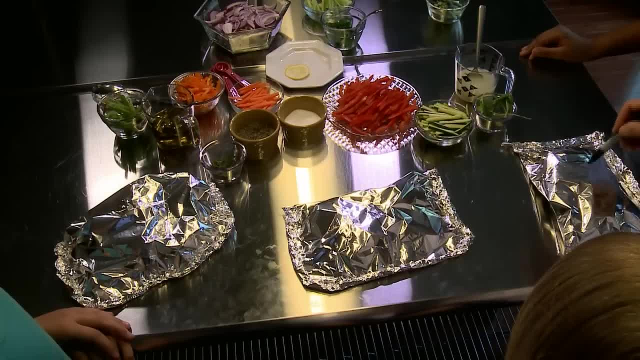 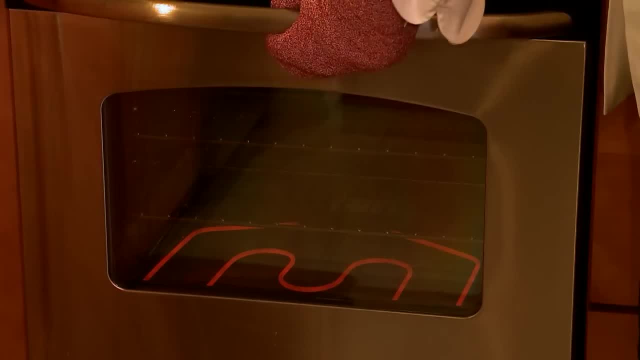 you can actually write names on the foil. Then when it comes out of the oven you'll know exactly which one is yours. The oven is set to 400 and preheated. We'll come back to check on them in 20 minutes and make sure the internal temperature has. 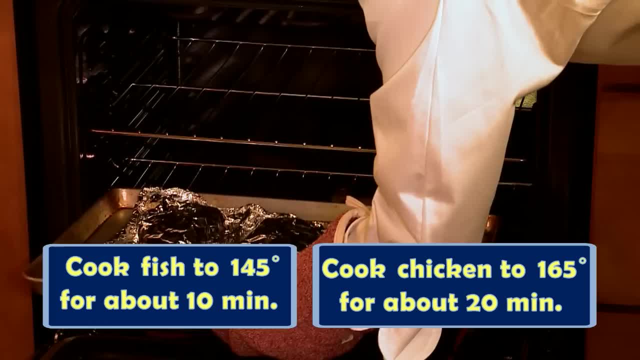 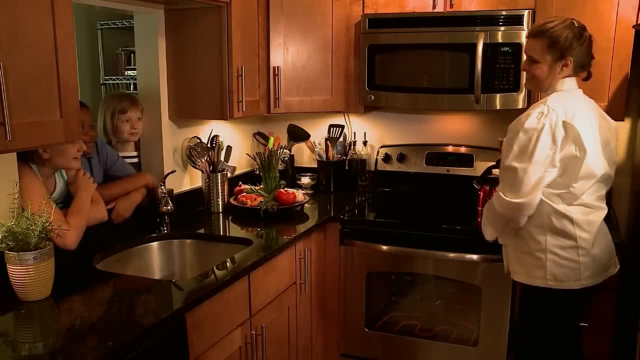 reached 165 degrees. So after 10 minutes we'll put the fish in. The fish will cook to 145 degrees internal temperature. While that's cooking, let's get started on the parfaits. We have some fruits here that you're familiar with, like strawberries, grapes, blueberries. 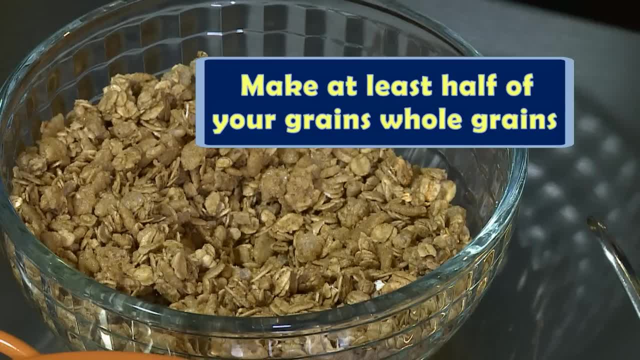 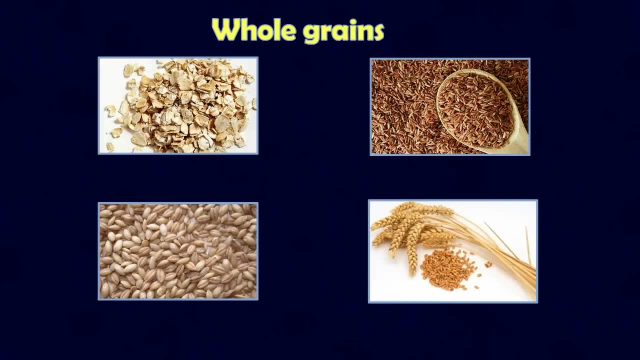 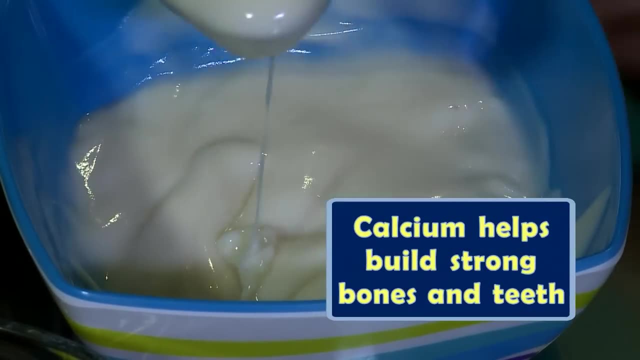 and bananas. For toppings we have some low fat whole grain granola and some pecans. Some examples of whole grain ingredients are oats, brown rice, whole grain barley and whole wheat. In our bowls here We have some low fat yogurt. Yogurt and milk sends calcium to your bones so you can grow up to be a strong young man. 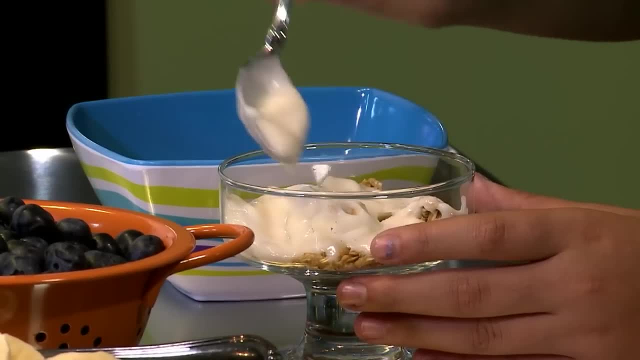 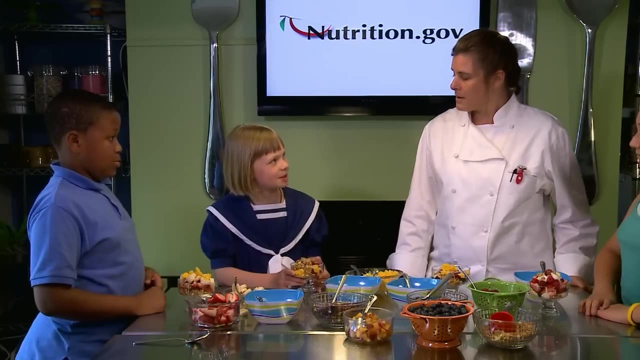 or woman in your case. How you do it is really up to you. Some people like to put the yogurt down first. Some people like to put the granola down first. I usually eat fruit for snacks, but sometimes I also eat them for breakfast. 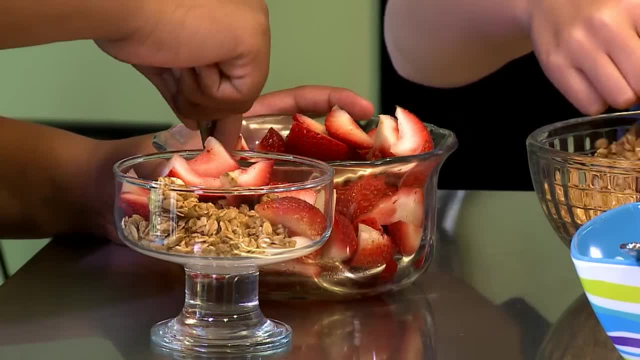 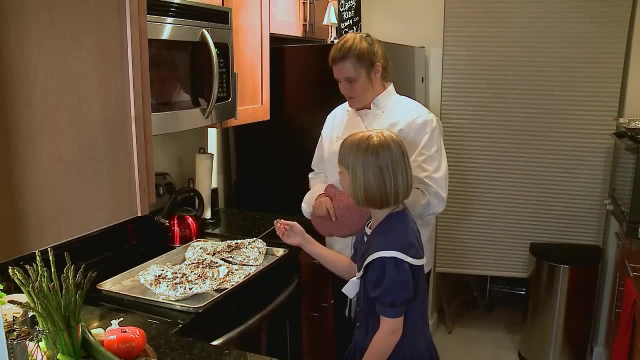 Fruit is a great snack. It can be good for breakfast, lunch, part of a meal or dessert. Here you go. Do you remember what temperature it should be? About 165 degrees, Perfect, Yay, it's done, Let's go eat. 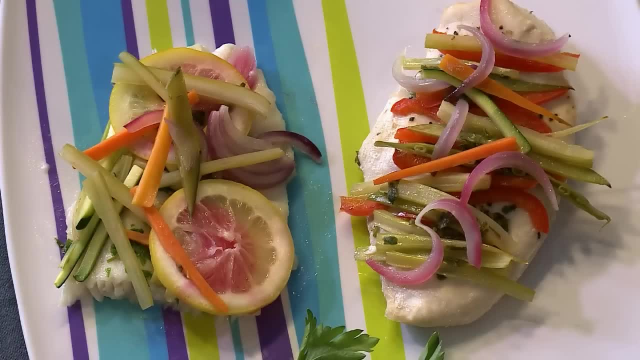 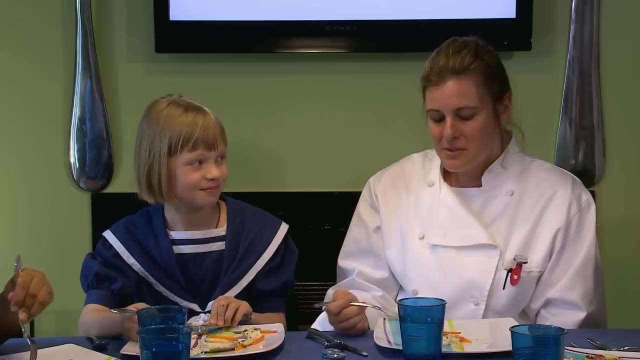 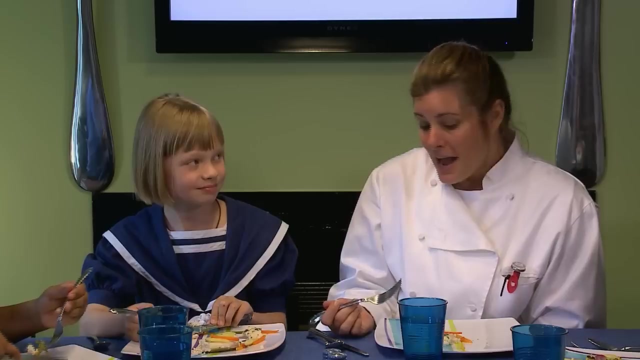 So here in this meal we have the protein from the chicken and the fish, and we also have all the vitamins and minerals from the vegetables that we've used. So my favorite part was working with you guys to put our packets together and creating our own unique flavors and now getting to taste how it comes out. 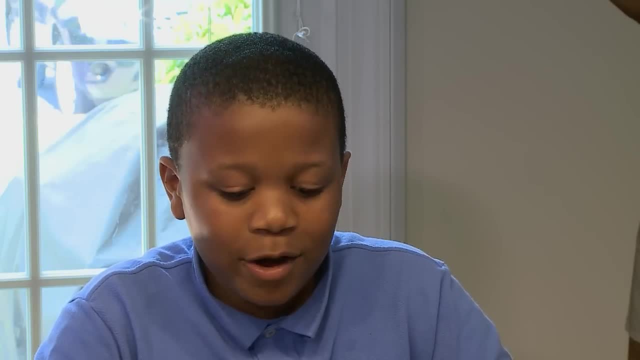 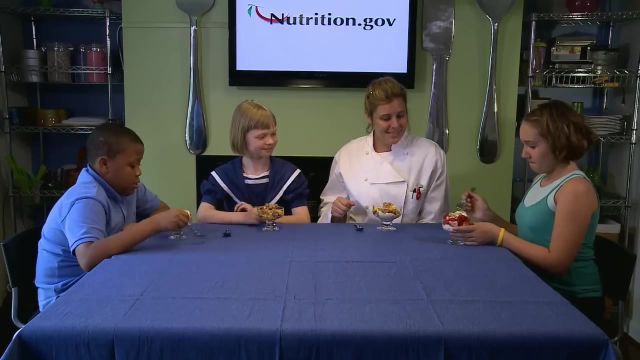 Yeah, it tastes delicious. The stuff is like edible art: It's colorful and creative at the same time. I didn't know cooking healthy foods could be so nutritious and fun. On to the parfaits, I can't wait to dig in.